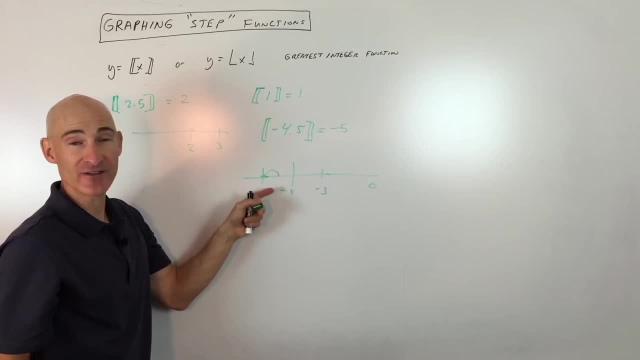 smaller than negative 4.5 because it's further to the left on the number line. Okay, so, are you with me so far? Okay, so the next thing is we're going to talk about how to graph these step functions. The first thing I would recommend doing is let's just make a table of values. So what I'll 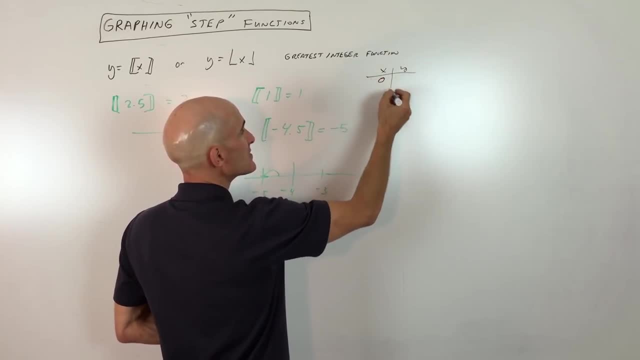 do is make a little table. I'm going to pick some integer values Like zero, that's going to round down to zero 0.5, that rounds down to zero 0.99,. still, zero. 1 is going to be 1.. Okay, 1.5, we round down to 1.. 1.999, we round down to 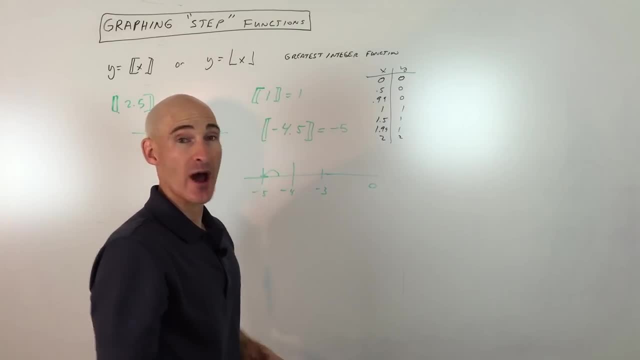 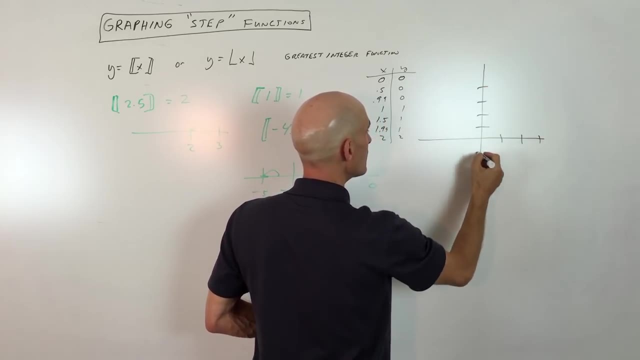 1.. But 2, we're going to be at 2.. Okay, and so on. So if we plot these points, okay, let's see if we can draw this here. 1,, 2,, 3,. okay, You can see 0,, 0,. that's going to be right. 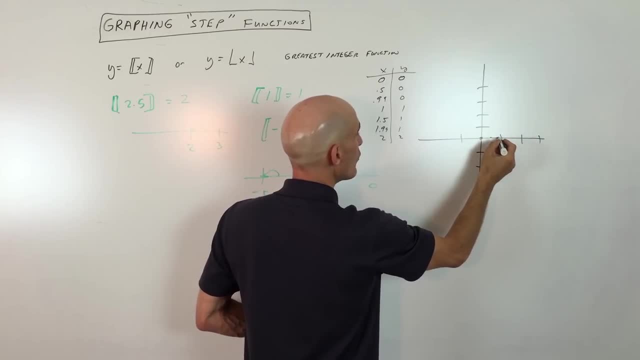 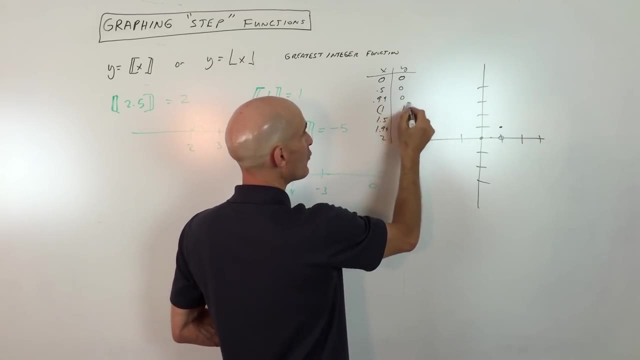 here 0, 0,, 0.5 is going to be right here 0.. 0.99,, that's 0.. But as soon as we get to 1, okay, we jump up to 1.. See, this is the .11.. So what we have here is we have a step, So you. 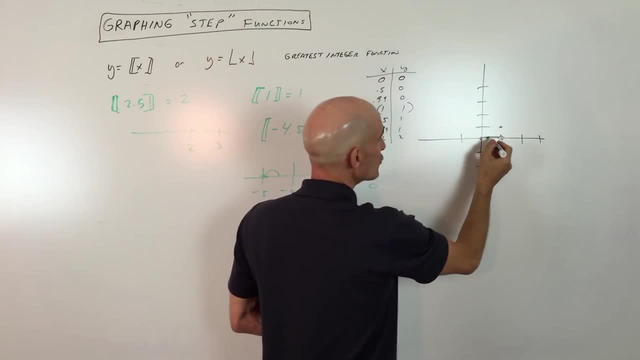 can see where it's. you know where the step function name comes from. Okay, so you go up to here. you jump up to 1. 1.5,. you're going to be at 1. 1.99, you're going to be. 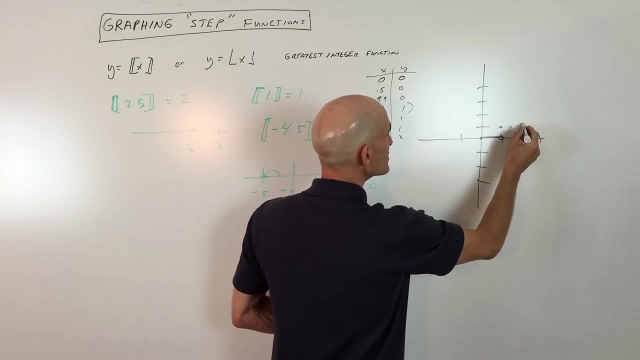 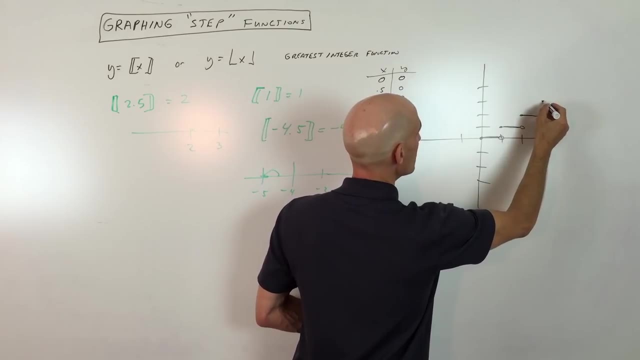 at 1.. At 2, there's an open circle here, right, because it jumps up to the next integer. Okay, so that's the next stair, And once you get a few of these stairs or steps going, you can repeat the process, okay. 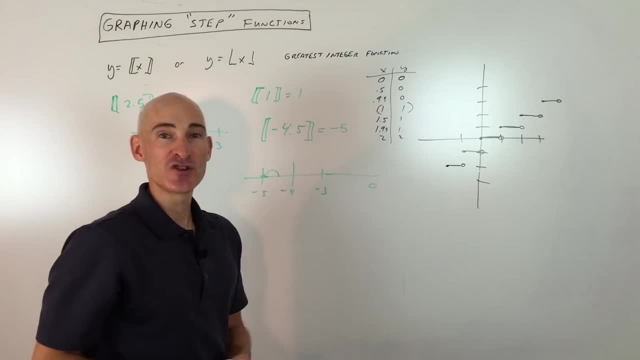 you know like. so both directions All right, so you're with me so far. Now this is a function because it passes the vertical line test. Notice like: right here it's open here, closed here, so it's only crossing. 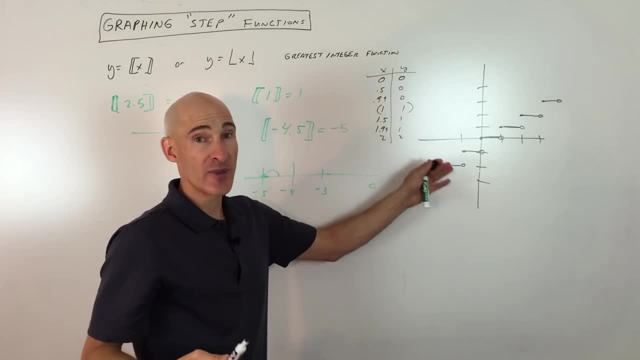 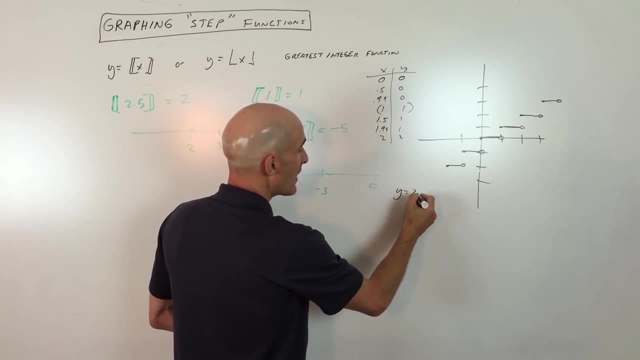 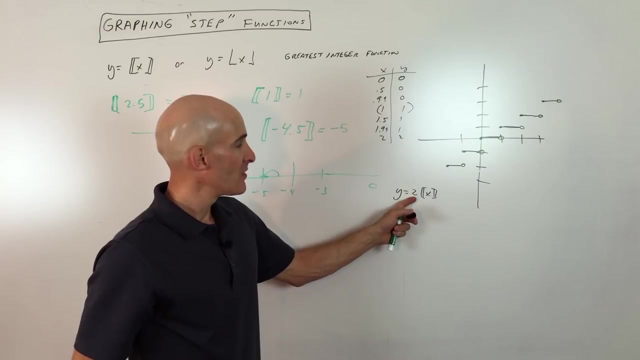 the graph at one point. So this is how you graph the basic graph. Now I just want to show you how to do a couple transformations of this function here. So say, you wanted to graph: y equals 2, okay, like this two times. What do you think this 2 does to the graph? Well, if you said that, 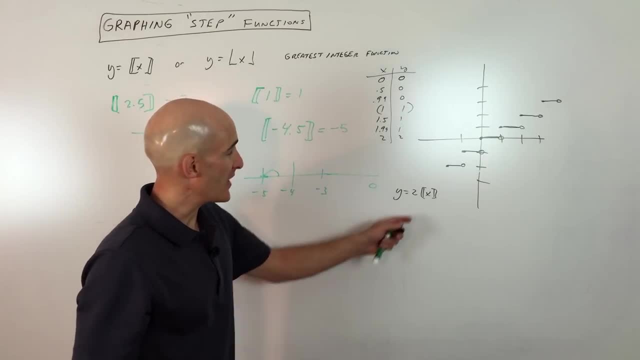 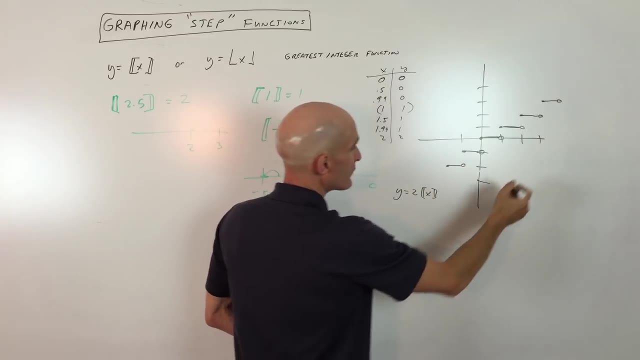 it stretches it vertically by two times. you're absolutely right. So, basically, what this is going to happen now is, instead of these stairs being going up one each time, they're going to go up two. Okay, so if I can sketch that, let's see, I'll put it right down here. It's. 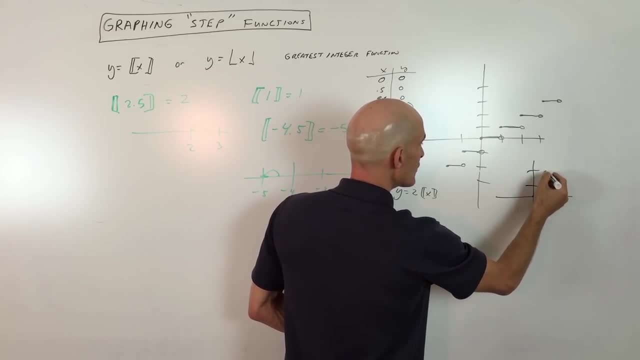 going to look something like this: now You're going to jump up to 2,. then you're going to jump up to 4.. Okay, and here you're going to jump down to negative 2.. Okay, so you're going to go up to 2.. Okay, and here you're going to jump down to negative 2.. Okay, so, 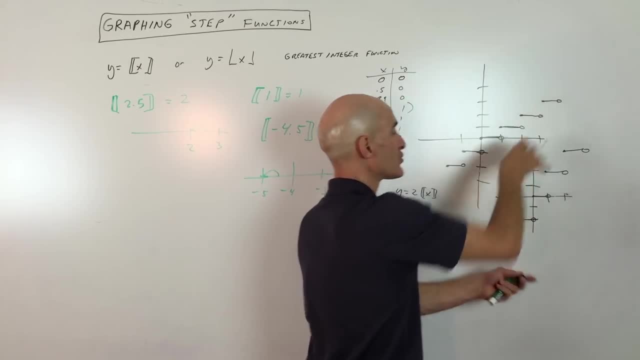 you're going to jump up to negative 2.. Okay, and here you're going to jump up to negative 2.. So it's a vertical stretch by 2.. So we're multiplying all the y values by 2.. Now what? 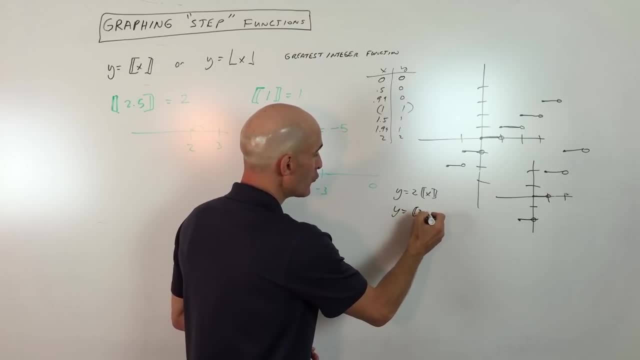 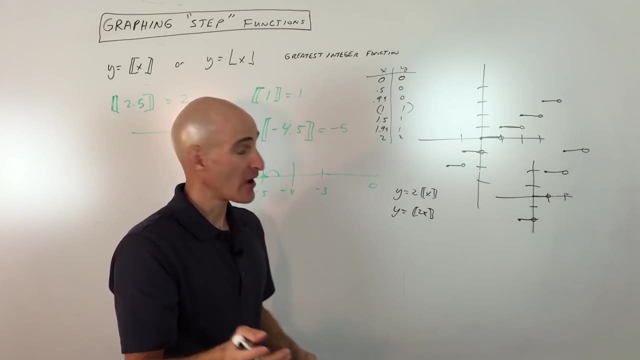 would happen, do you think if I put the 2 grouped, okay with the x? Well, if you said that it's going to be a horizontal compression, you're absolutely right. The thing to remember is that when it's grouped with the x, it has the opposite effect. Okay, so for another. 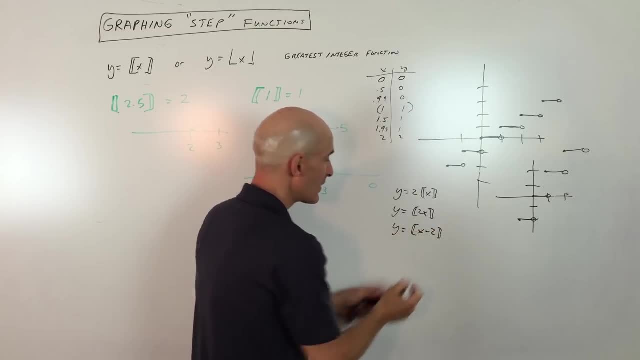 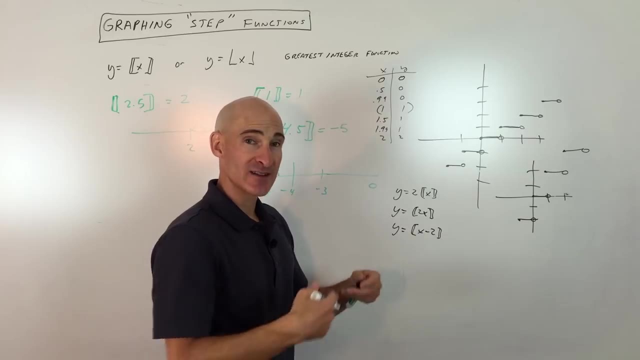 example like: say: for example, we have x minus 2.. You see the minus 2, and you might, might naturally think: well, minus two means left, two right, but when it's grouped with the x, it has the opposite effect. this is actually going to shift the graph right too, so you're going to pick the 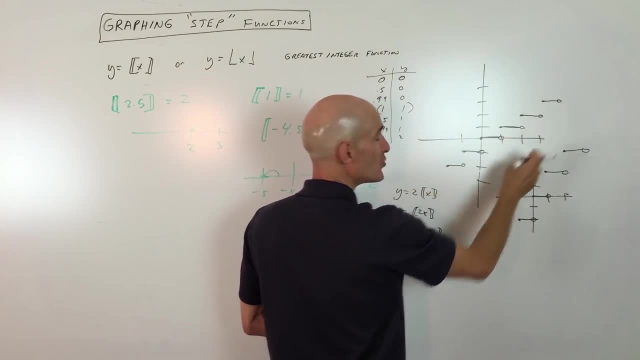 graph up. okay, this graph here, pick it up. you're going to shift it two units to the right, whereas this one here we're just going to multiply all the x's by one half, and so what's going to happen is it's going to compress it horizontally, so these stairs are actually just going to be. let's see if. 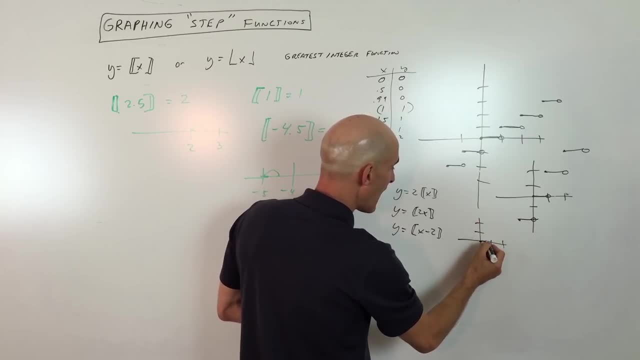 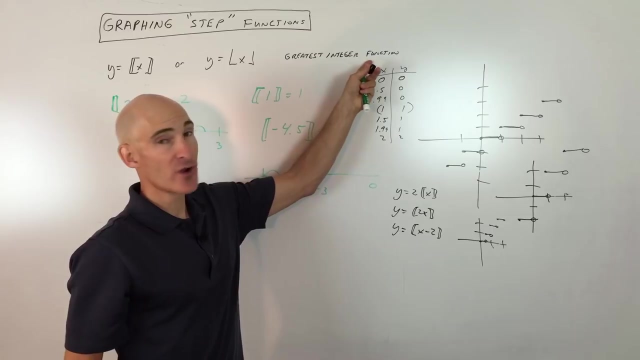 i can sketch that here for you. they're just going to be like half, then it's going to jump up to the x one, okay, like that. so basically it's compressing this way. so i hope this helped you to understand how to graph the step functions. okay, also known as the greatest integer function. take a look at. 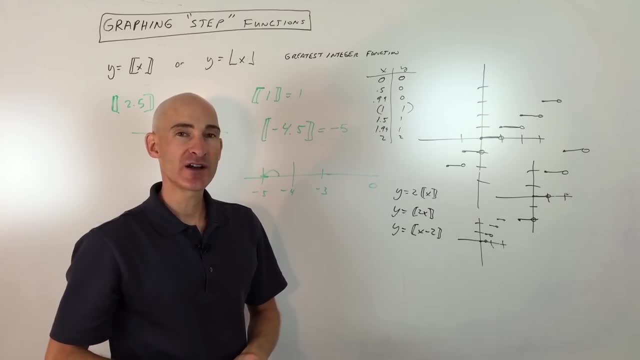 some of these examples here, and i'll also have a video that talks about the different transformations that we're talking about here. if you want to learn more about that- and i can put a link for that for you- so subscribe to the channel. check out some of my other videos on mario's math tutoring youtube. channel and i look forward to seeing you in the future videos. i'll talk to you soon.